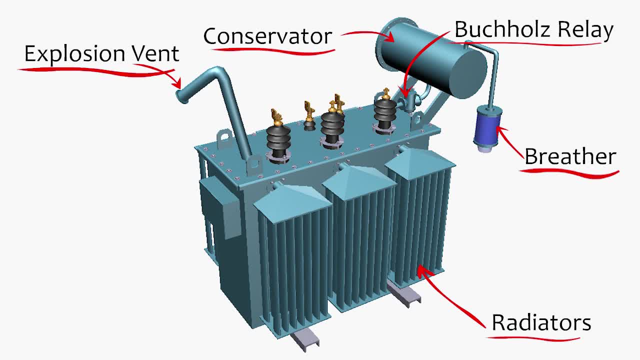 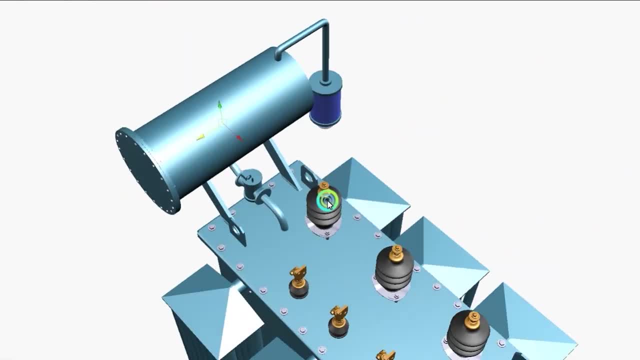 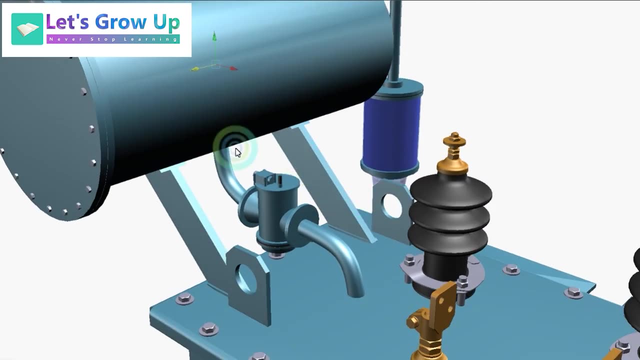 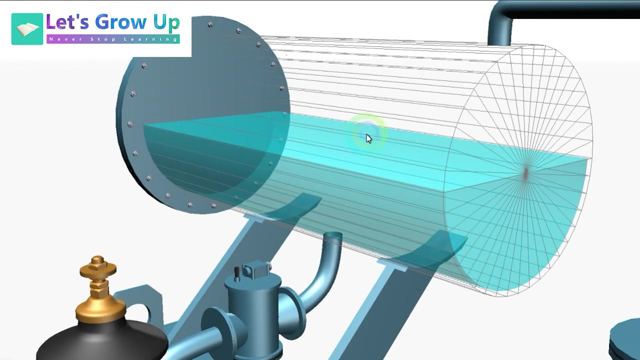 the all components and its working principle. Let's see the conservator tank. It is a small tank which is used in high power transformer- Only for high power transformer. you can see it. So it is connected above the main tank. The main tank and the conservator tank are connected to each other through a pipe. The working of the conservator tank is very simple. Look, the 50% part of this conservator tank is filled with oil and the other 50% is 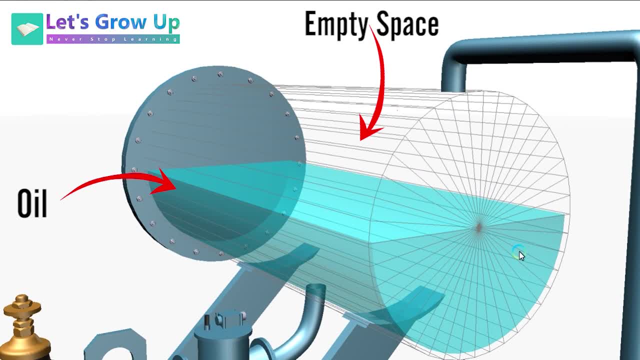 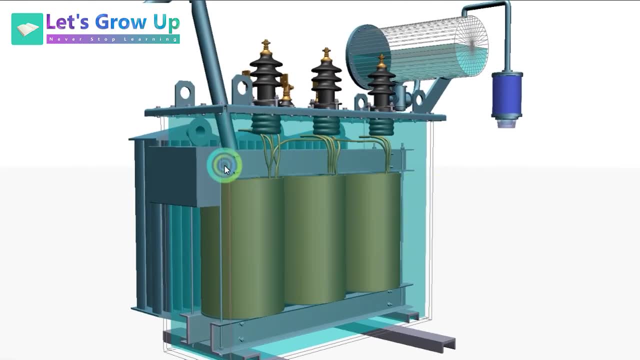 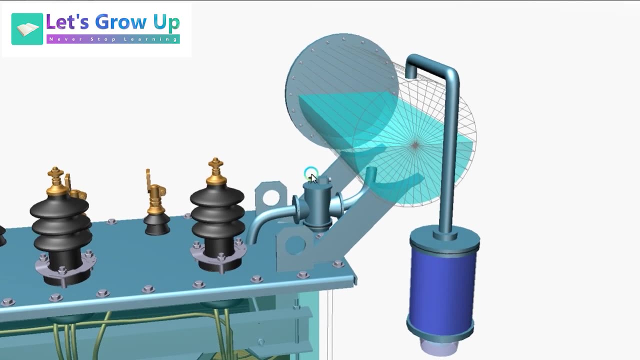 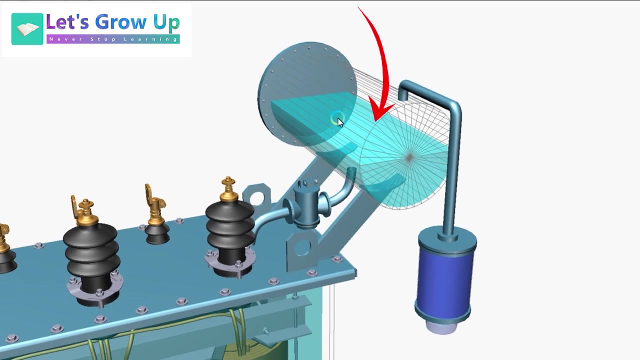 empty or it is a gap. and in this gap you know that the transformer tank is filled with oil and the during the working of the transformer it created or it produces heat. So if the heat level is extreme level, at that time the oil try to expand. So that time needs extra face. So this space, this space used at that time, and keep the transformer safe, Right if there is no extra face. 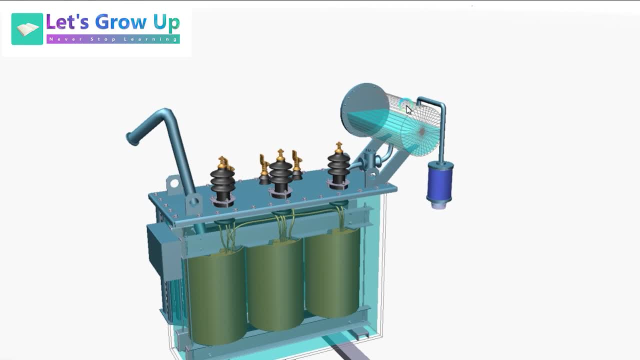 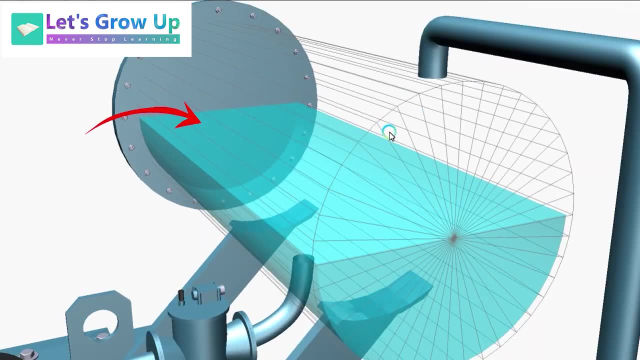 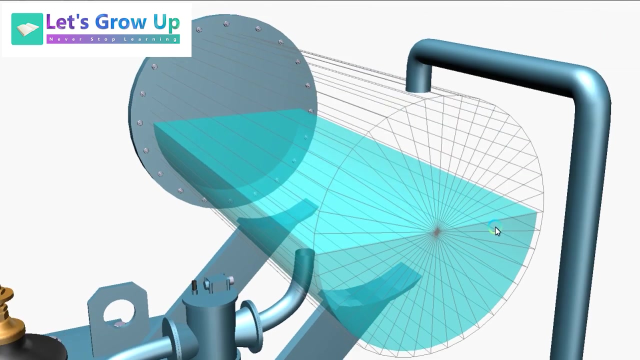 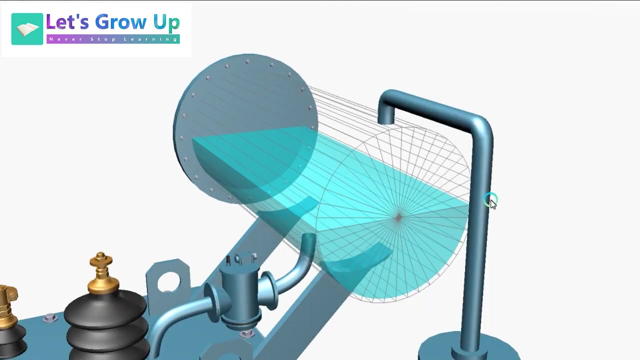 the oil. try to expand, Try to expand it, but there is no extra face at that time, So it will blast Right. So need space to expand the oil. That's why the conservator tank: there is extra face, Okay, And the space is filled with air. The space is filled with air. Obviously there is a gap. The gap is cannot empty. Breather is a device which is used for breathing of transformer. 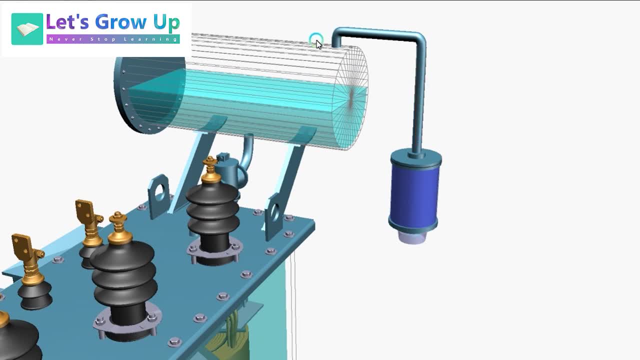 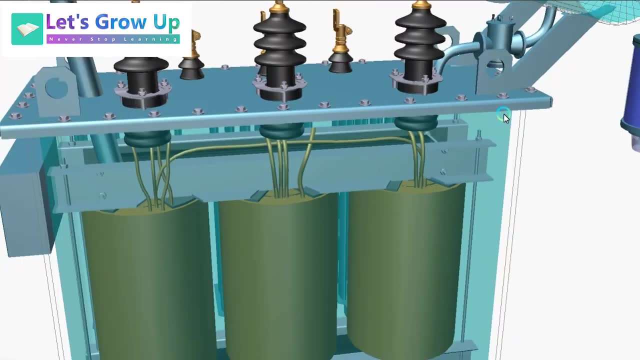 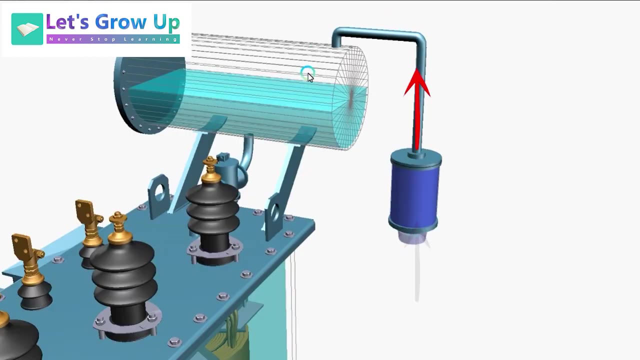 It means air goes in or out from the transformers. So when the hot oil expands, air goes out from the transformer and and when the oil contracts after cooling, the air enter the transformer. Okay, Normally the incoming air may be consist of moisture and dirt and it may be causes of damage inside the transformer. Different types of damage may be. So that's why the silicon 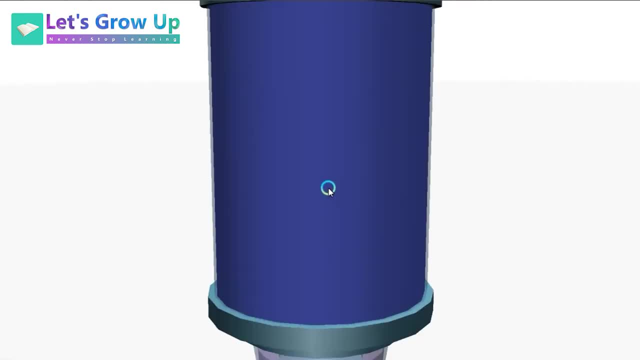 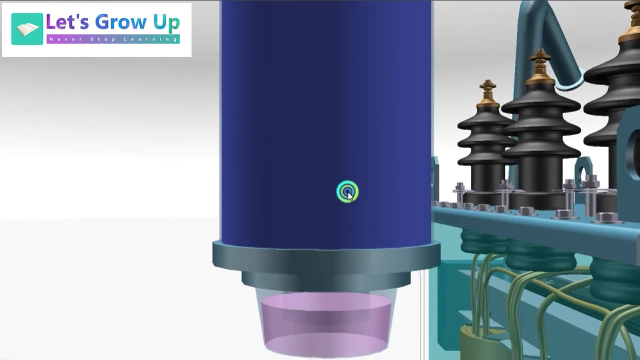 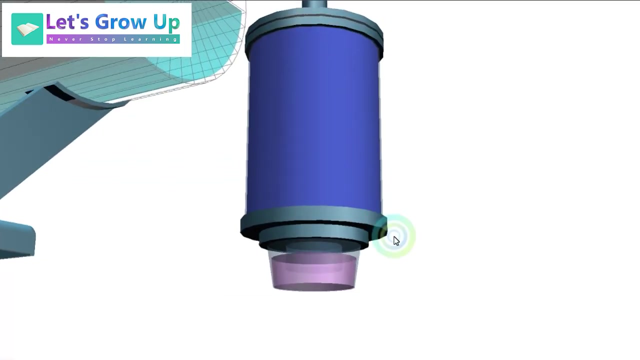 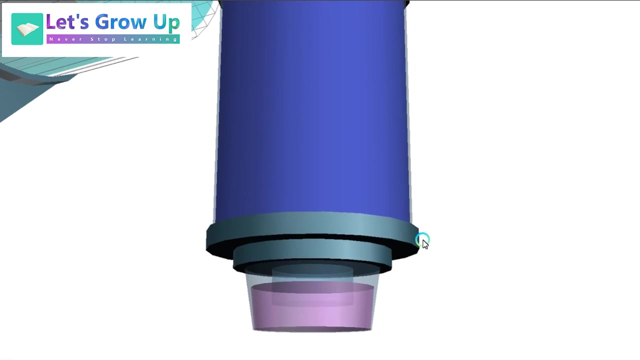 is used inside the breather. When the air enter the enter the transformer, through this breather the silica gel absorb the moisture. only dry air enters into the transformer. So here you can see this breather also have an oil cup fitted with so that the dust particle gets settled in the cup. Okay, So oil is used for dust, So silica gel used for moisture and oil is used for. 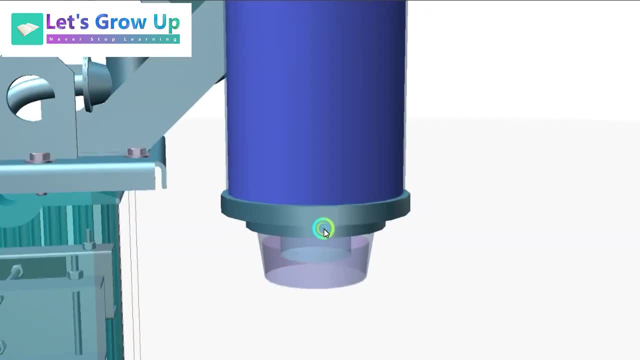 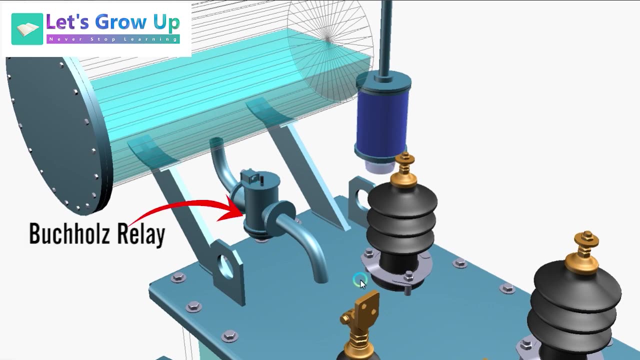 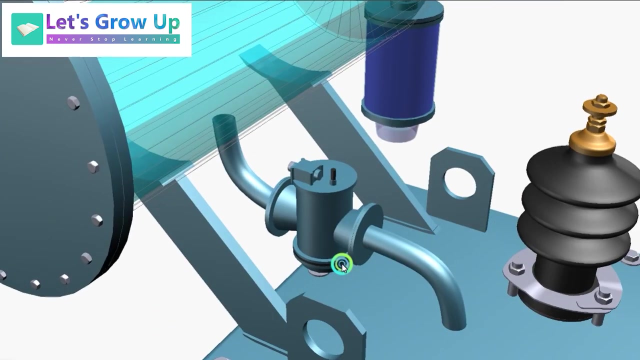 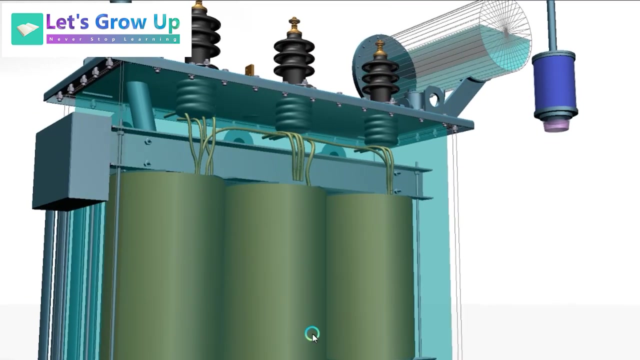 dust. Okay, Both are. both are clean by this process and only dry air can enter in the transformer. Next is Bukoji relay. It is placed over the connecting pipe that runs from the main tank to the conservator tank. The purpose of this device is to give the protection to a transformer from the different faults happening in the transformer, like short circuit, inert, run core, incipient, etc. If there is any fault inside the transformer, 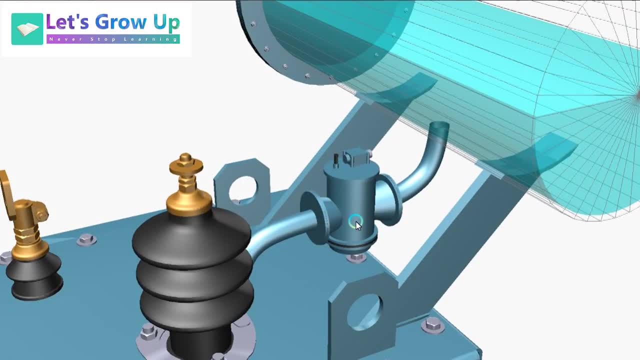 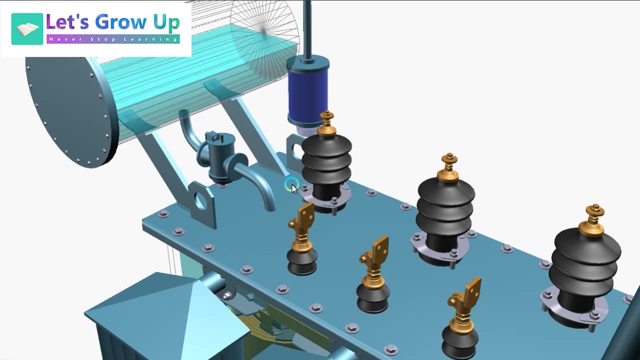 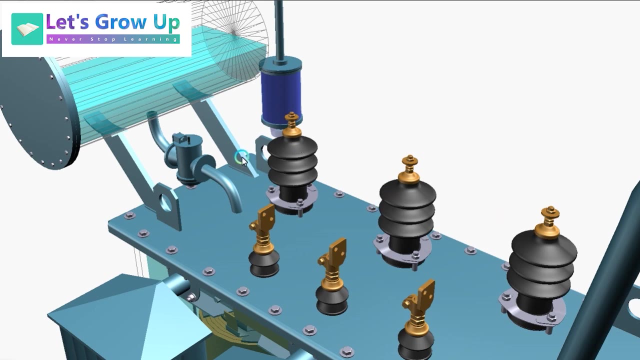 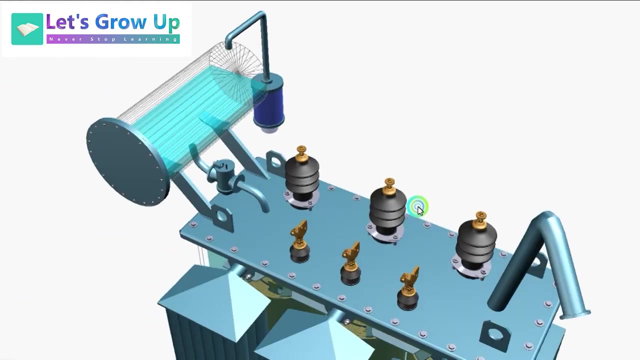 so it automatically switch off the transformer or shut down the transformer. Okay, Just like a. you can think it. just like a NCB, NCB also same process work. So I will make make a video particular how the Bukoji relay work. Okay, So it is a technical part, So I will explain it with another video. Next part is radiator. The radiator of the transformer accelerates the. 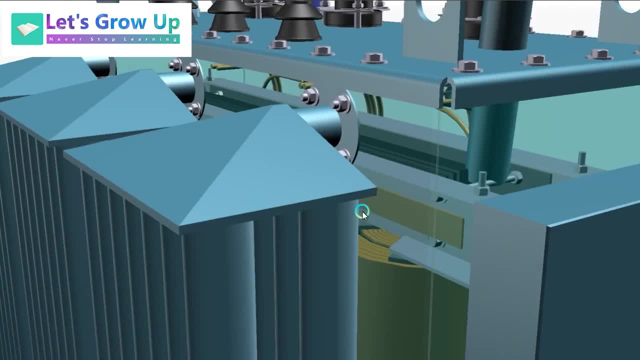 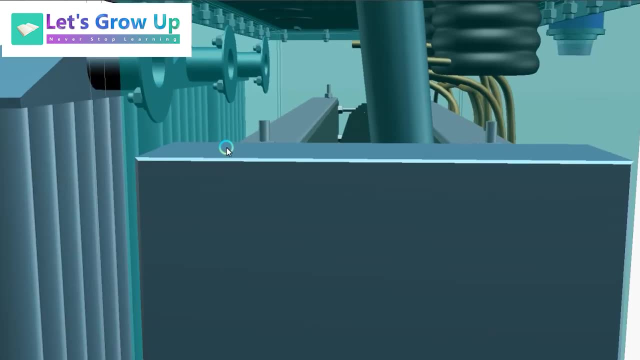 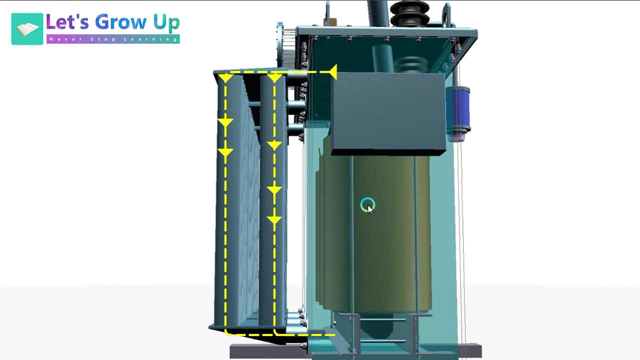 cooling rate of the transformer. Thus, it plays a vital role in increasing the loading capacity of the electrical transformer. This is the basic function of the radiator. Okay, So I am sharing an animation so that you will get the idea the how the radiator work. Actually, inside the radiator there is very small, more thin, thin pipe. Okay, When a transformer is loaded, the current is following through its winding The radiator of the transformer accelerate the cooling rate of the transformer. 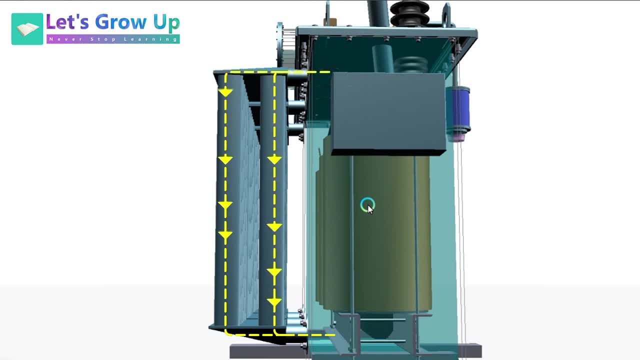 more. okay, so it is the basic method of radiator. so you can see this animation so that you will get the idea. the how does the how does the radiator works, the main work of the radiator: the hot oil inside the tank passing through its own pipe, so that when the passing the oil 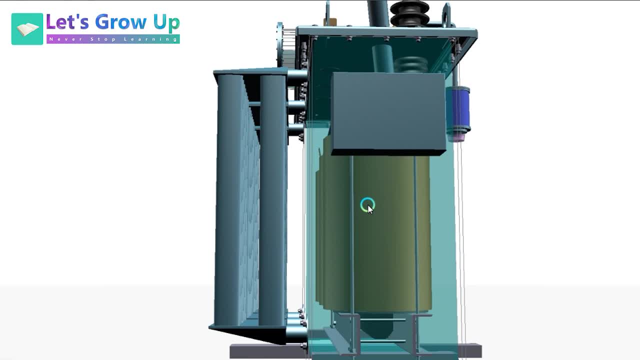 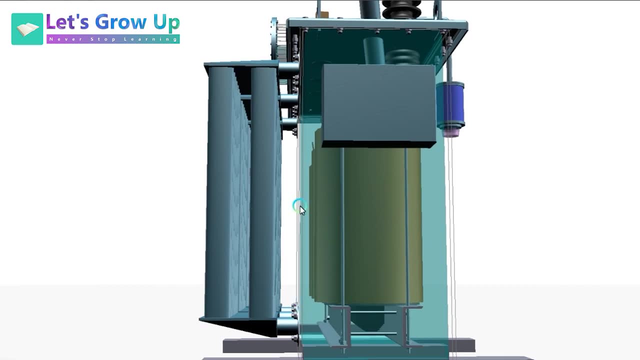 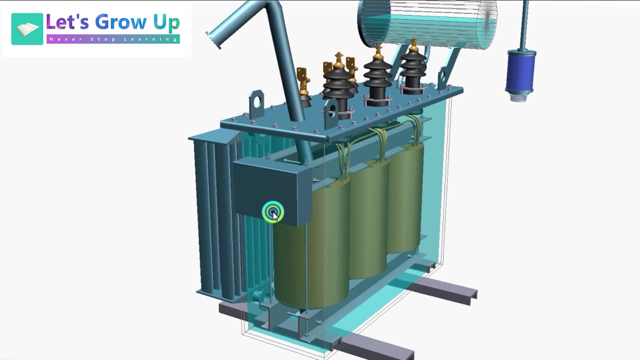 through a long distance. automatically it will reduces the heat and again cool the oil. and this cycle happens again and again inside this radiator. okay, so that's why it accelerate the transformer cooling system. so also there is conservator tank to expand the oil. but if there is any danger level, 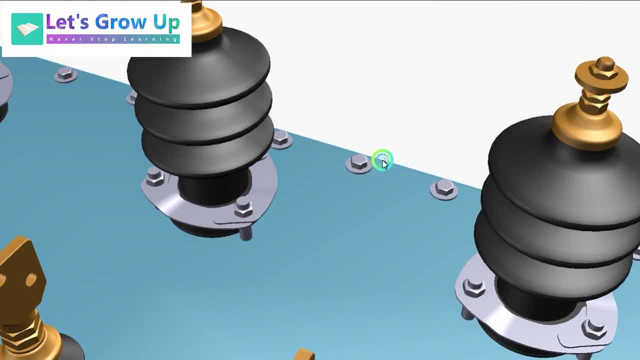 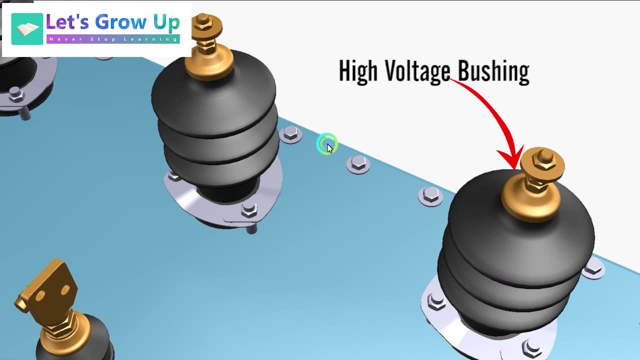 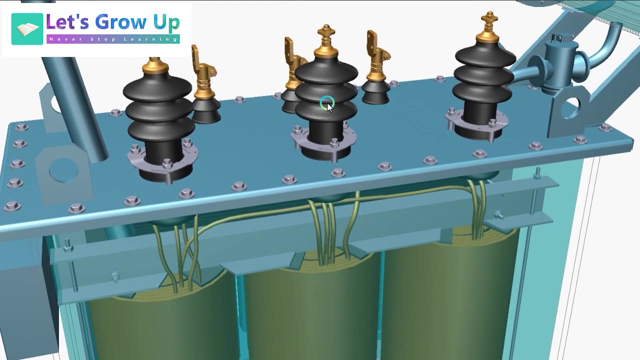 so this radiator also works side by side. okay, bushing, so next is bushing. bushing are used to bring winding terminals out from the tank and also used for insulation, for example. so there is there is two type bushing. one is lv- low voltage bushing, or you can see this. 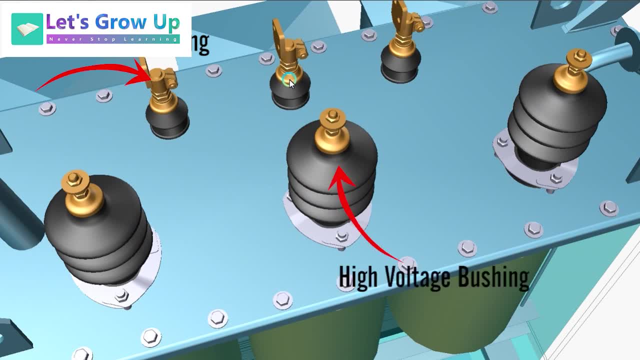 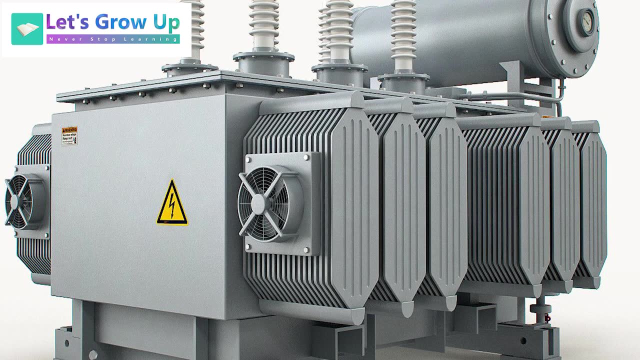 it is a hv high voltage bushing. also you can see some transformer cooling fans. the radiator is used for cooling system, but also there is cooling fans, some big transformer like 26 mba and the above transformer cooling fans are also used on radiator. so you can see this. 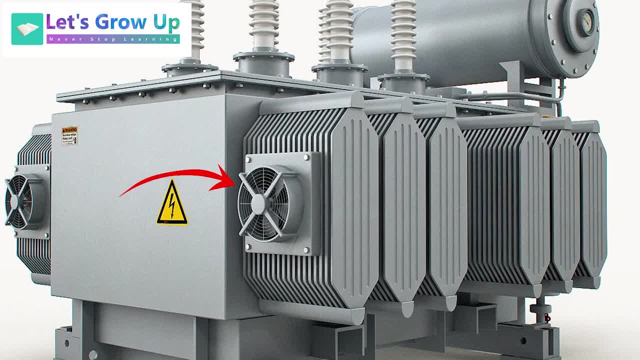 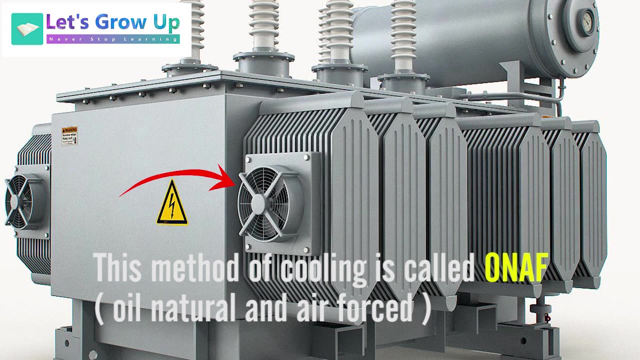 image. the radiator fan is used. okay, oil temperature gauge provide on or off signal for the cooling fans. when the temperature becomes generated more than 75 percent, the temperature oil gauge turn on the cooling fans and the method of the cooling is called the o? n a f: oil, nature and air forced. so 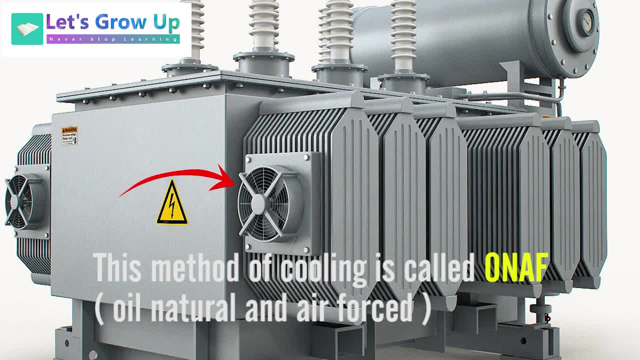 oil, nature, air force. we will learn the type of transformer, okay, the cooling system based on the cooling system. the cooling system is based on the cooling system based on the cooling system, different type of transformer. so it is a. it is a copy, so if there is any very good feedback from all, 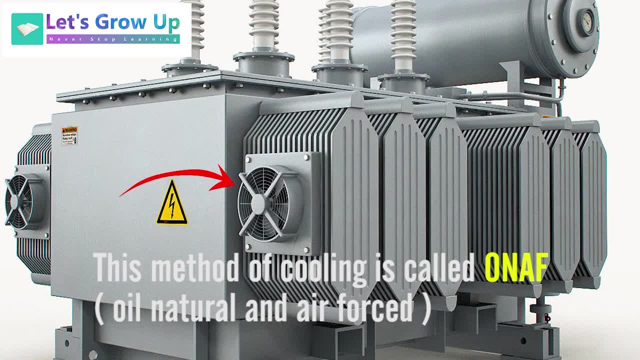 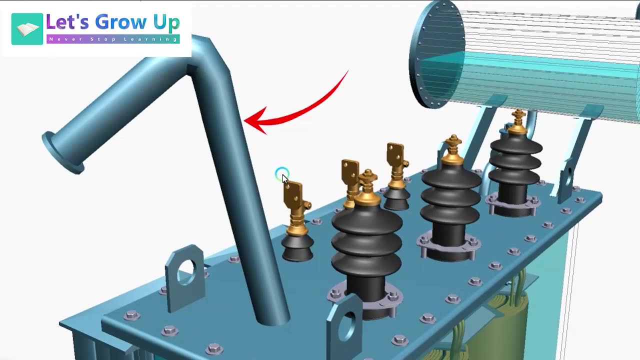 of you. i will make another video type of transformer based on their cooling system. there are different types of transformers, so o n a f is a one type of transformer. okay, if i get very good feedback for this video, i will make another video, obviously, okay, the last is explosion vent. okay, explosion vent, or. 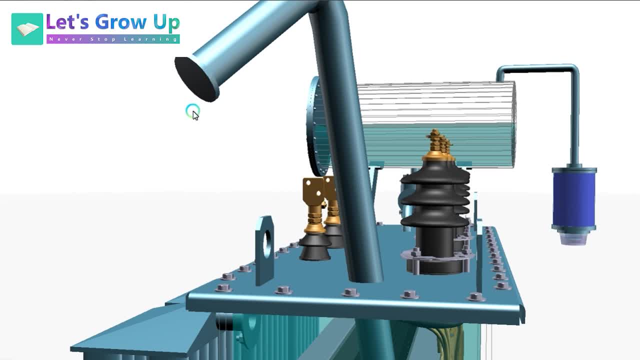 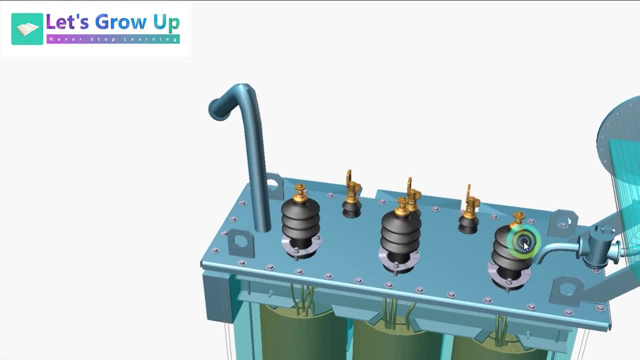 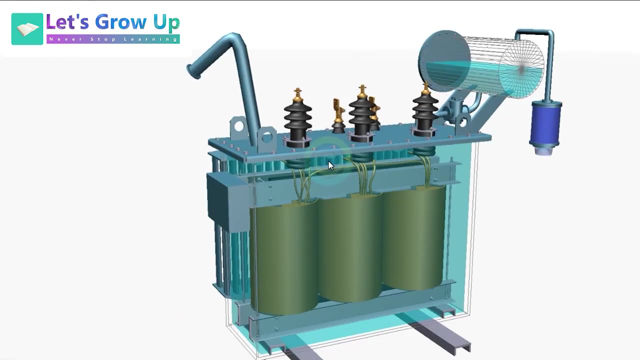 style of the theo cap is used to make a bras iulian transformer. okay, next of all, we okay. so it is the last part. if the all devices are fulfilling, there is no way. there is no way, then the explosion vent. so the main problem of the transformer is heating problem. so there is. 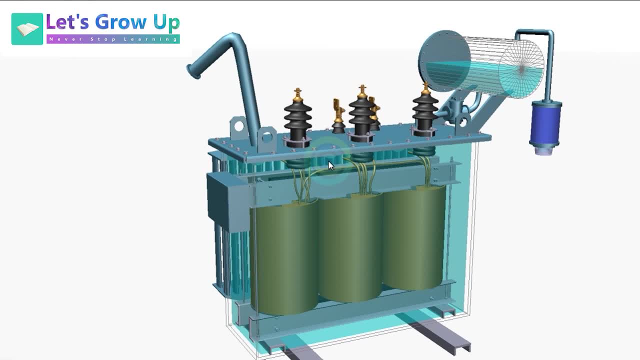 a oil, if the oil temperature is too much hot, just like you can think, when we regularize afteraman, solar thermal pump is used. this is a solution of the transformer, to the energy efficiency of the transformer. so if the oil temperature is too much hot, just like you can more or less kill the heat you can use''.